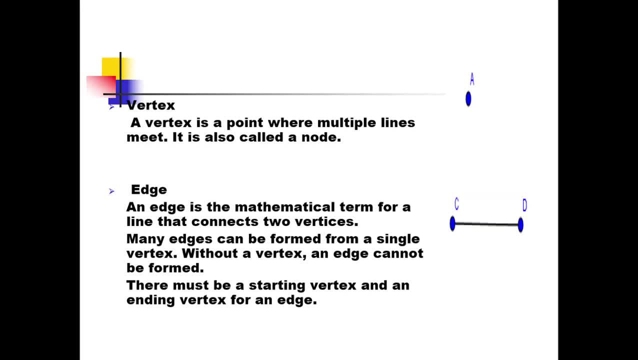 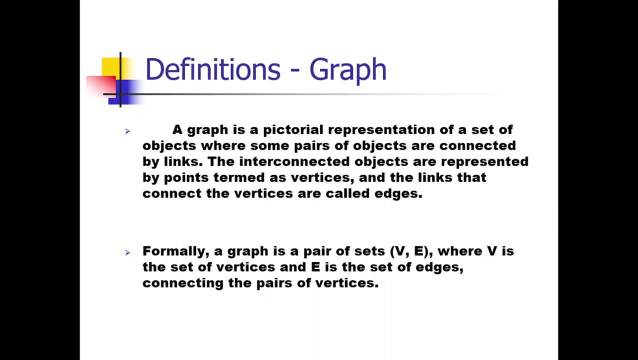 So it is the definition of vertex and edge. Without a vertex we cannot define the edge, We cannot draw the edge there. So to creating any graph, You should have at least one vertex. that So definition of graph. So graph is a pictorial representation of a set of object. 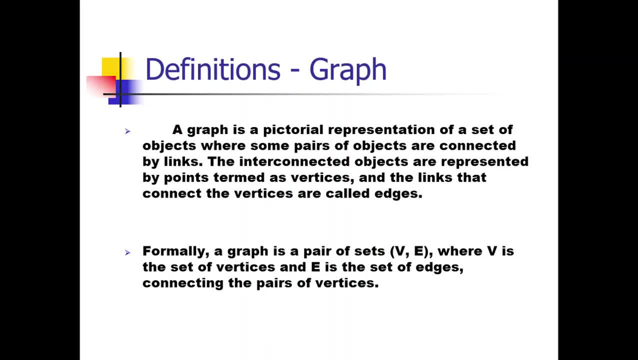 Where some pair of objects are connected by link And the interconnected object are represented by point That is called a vertex And the link that connect the vertex that is called edge. So it is a pictorial representation of set of objects. In this set of objects they consider the vertex and edges. 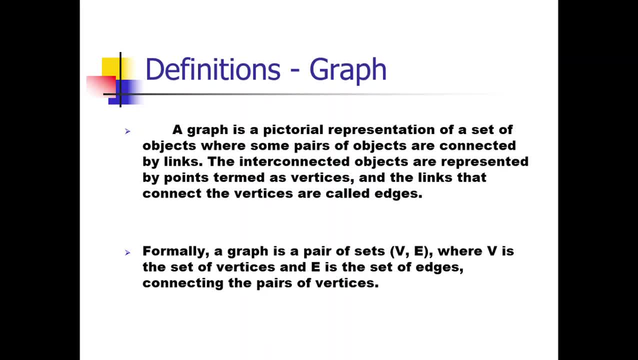 Where the vertex connect by the link And that is called the edge. Formally, a graph is a pair of set, VE, Where V is a set of vertex and E is a set of edges Connecting the pair of vertices. So it is the definition of graph. 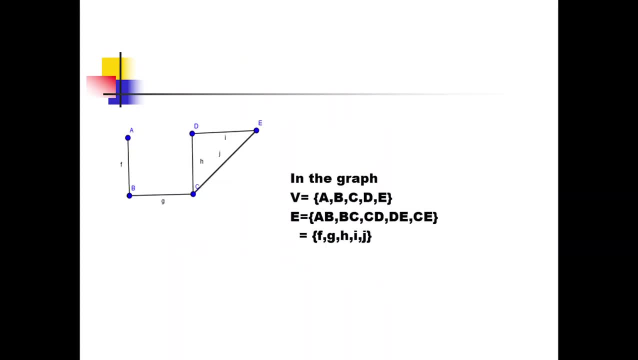 So this is the example of graph here. In this graph there are five vertex. are mentioned A, B, C, D, E. That is arbitrary notation here. Arbitrary name: You can use the V1,, V2,, V3,, V4, V5 notation. 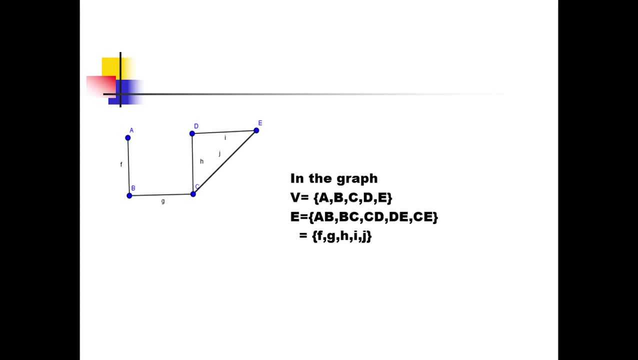 And the edge is a connection between the two vertex, That is the F, connection between the A, B, That is the B, C. That is the edges of G, H, I, J. So these are the edges of this graph. 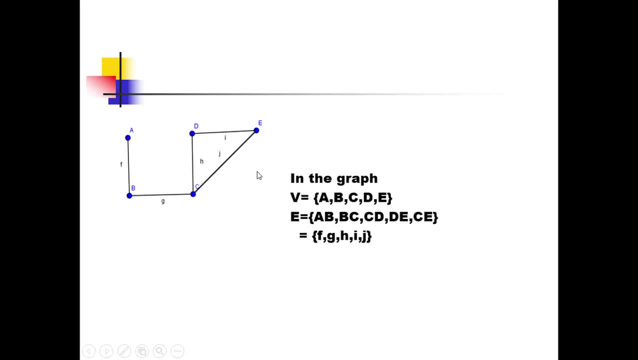 There are five edges in this graph And you can also mention the name E1, E2, E3, E4, E5.. So it is the example of graph. So next definition is a loop. So in a graph if an edge is drawn from vertex to itself is called a loop. 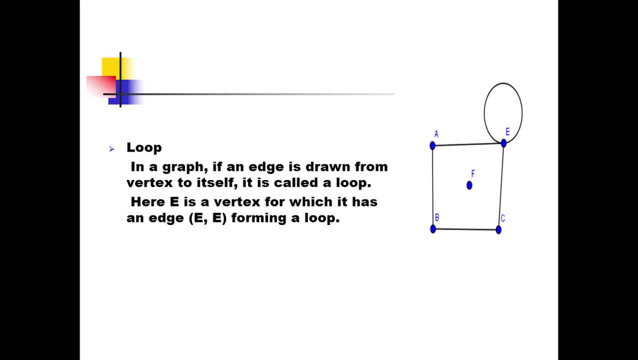 Here the vertex E, for which it has an edge E2, E. This edge is called a loop Because its starting and ending vertex are same. That is called edge Because its starting and ending vertex are different. So any edge which starting and ending vertex are same. 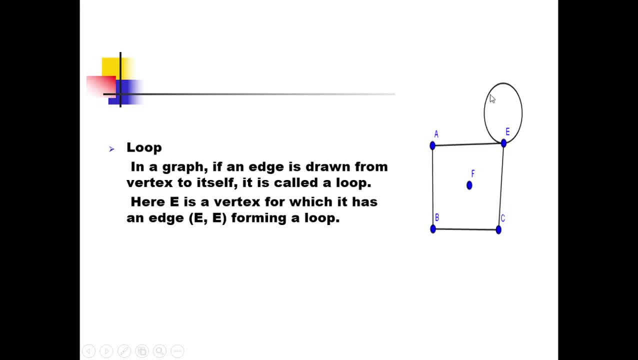 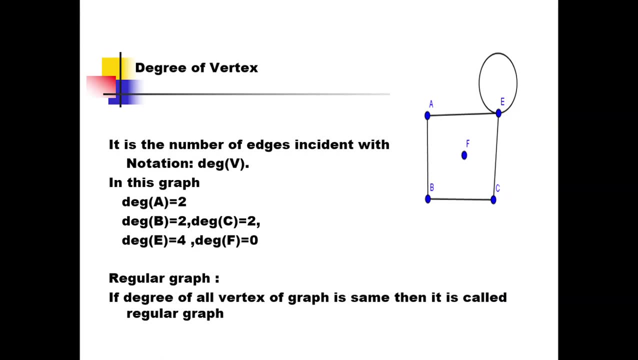 Starting and ending are same. That is, starting is E with ending is also E. So that is called a loop Degree of vertex. So it is the number of edges incidence with the vertex. It is the number of edges incidence with the vertex. 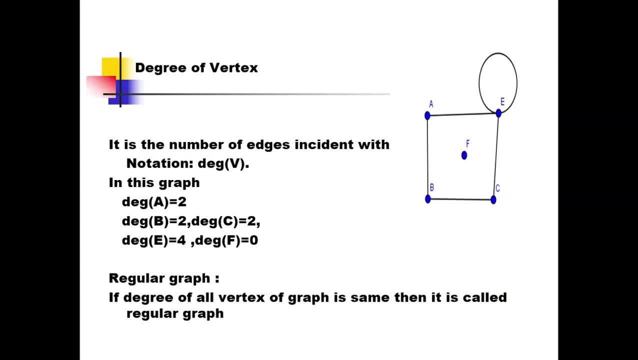 That is called a degree of the vertex. So here degree of A. There are two edges are incidence with A here. So degree of A is 2.. Degree of B is also 2.. Degree of C is 2. Because there are two edge are incidence that. 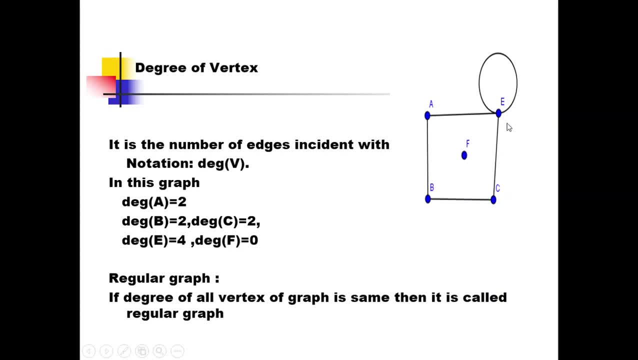 Degree of E is a 4.. Because there is one loop there, So degree of any loop is a 2.. And remaining are two edges, So degree of the E is a 4.. And F is a 0.. That degree of F is equal to 0.. 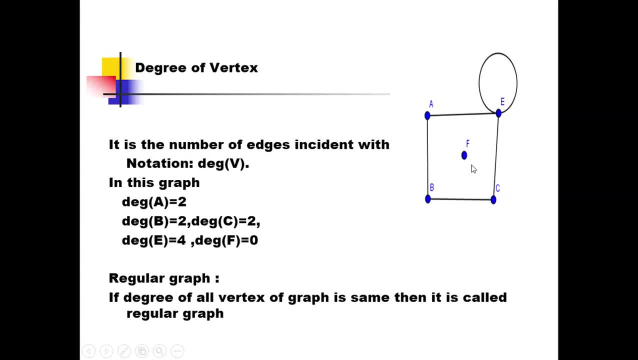 Because there is no any connections with the F. So that is called degree of vertex. Next definition is regular graph. If degree of all vertex of graph is same, Then it is called a regular graph. So this type of graph is known as a regular graph. 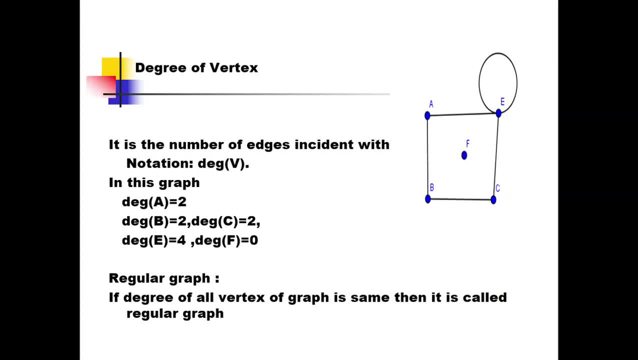 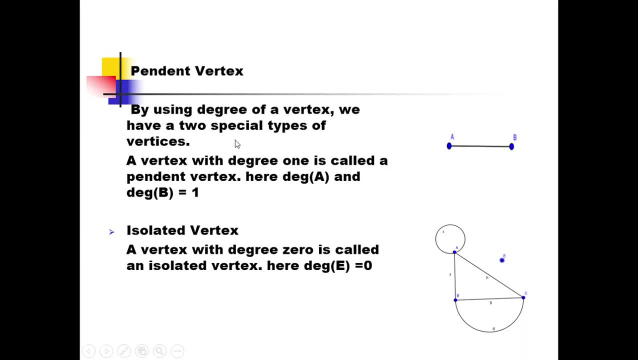 If all the vertex have degree equal, Then it is called a regular graph. Next is a pendant vertex, So a vertex with degree 1. That is called a pendant vertex. So your degree of A and B is equal to 1.. So any graph which consider any vertex with degree 1.. 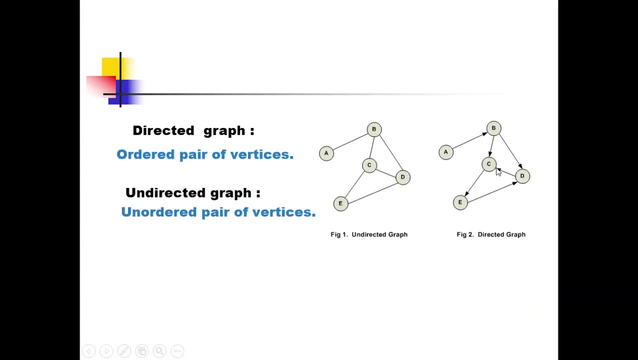 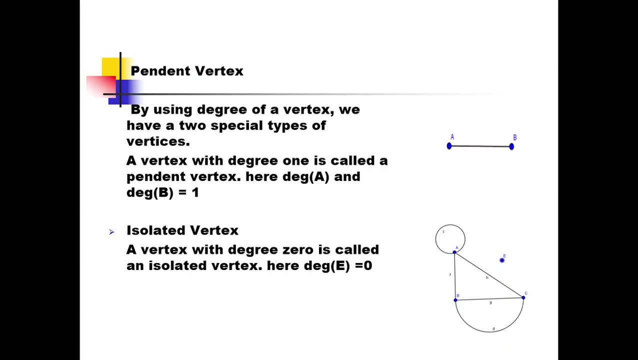 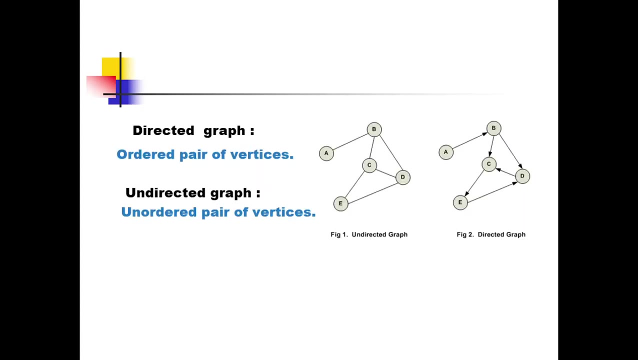 So that vertex is called a pendant vertex. Next is a isolated vertex. So vertex with degree 0 is called a isolated vertex. Here degree of E is equal to 0. So that type of vertex is called a isolated vertex. Next definition is a directed graph. 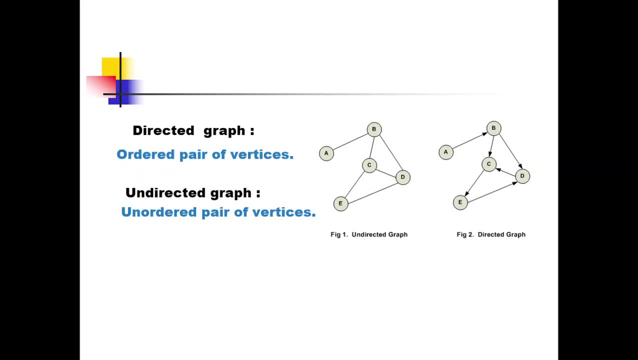 In such graph if direction is mentioned from F, From any two vertices, So that type of graph is called a directed graph, And if direction is not mentioned in such graph, That is called a undirected graph. In this first graph it is undirected graph. here. 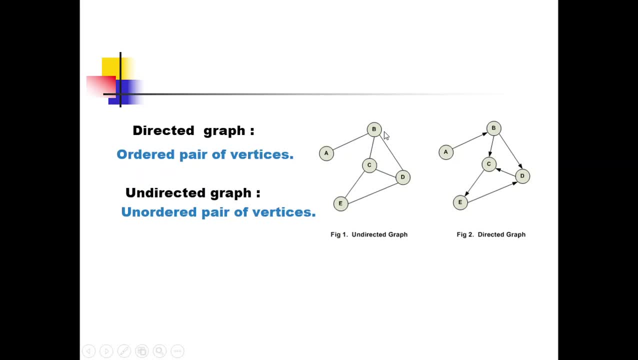 There is no any direction mentioned between A to B, B to D And remaining all that, So it is called a undirected graph And here, when direction is mentioned- that A to B There is a direction is mentioned And you have to strictly follow this direction. 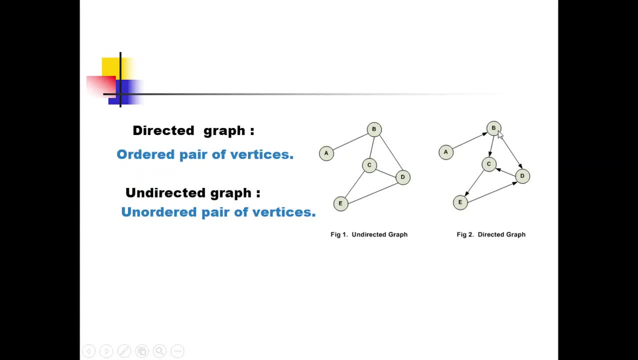 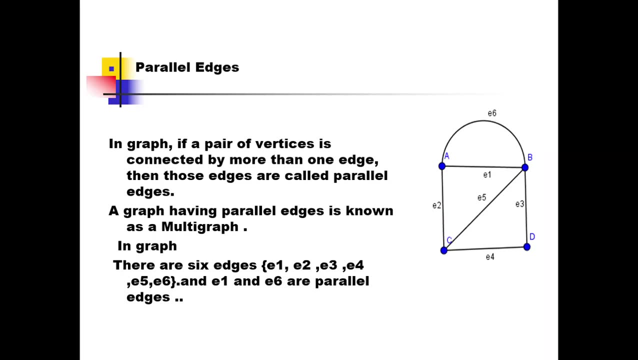 To reach A to B. So that is called a directed graph. Next is a parallel edge In a graph: if pair of vertices is connect by more than one edge And then those edges are called the parallel edge, So any two vertex that connect by more than one edge. 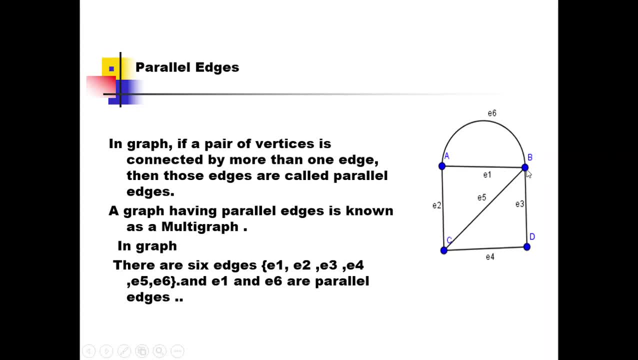 So here in this graph A and B are connect by the E1. As well as A and B are connect by the E6. Where starting and ending are same for both the edges. So these two edges are known as a parallel edge. 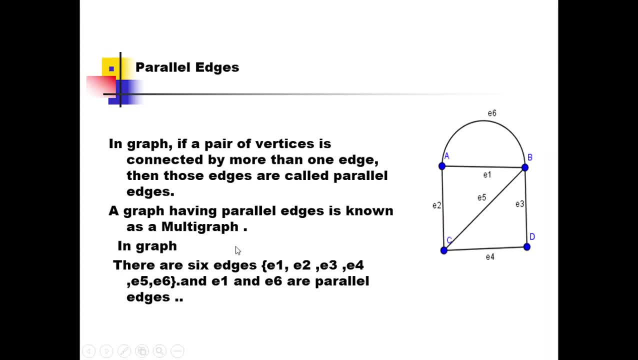 And the graph having parallel edge that is known as a multi graph. So that type of graph is called the multi graph And in this graph there are six edges: E1, E2, E3, E4, E5, E6.. 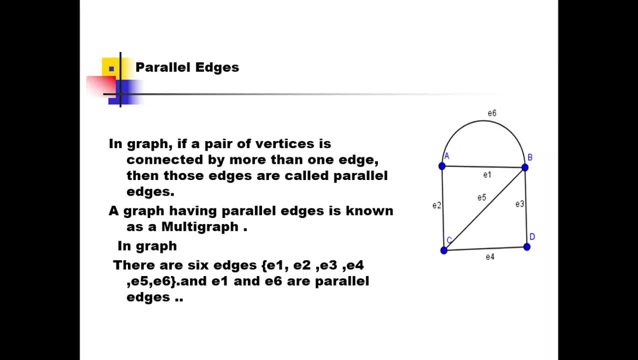 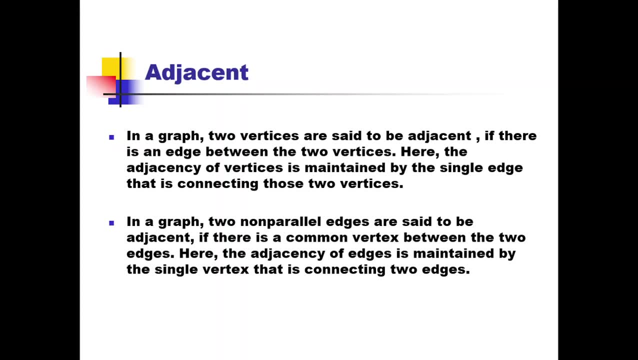 And where E1 and E6 are a parallel edges Adjacency. So in a graph two vertex are said to be adjacents If there is an edge between two vertices. And here the adjacency of vertices is maintained by the single edge. 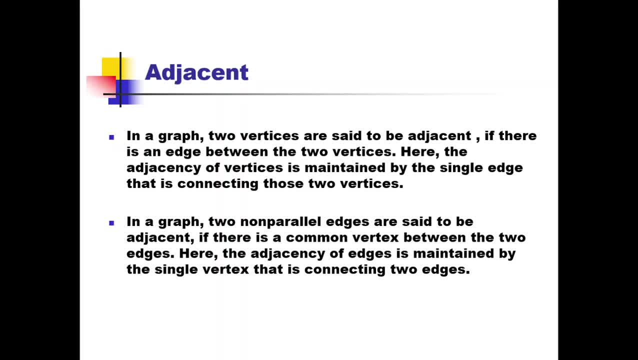 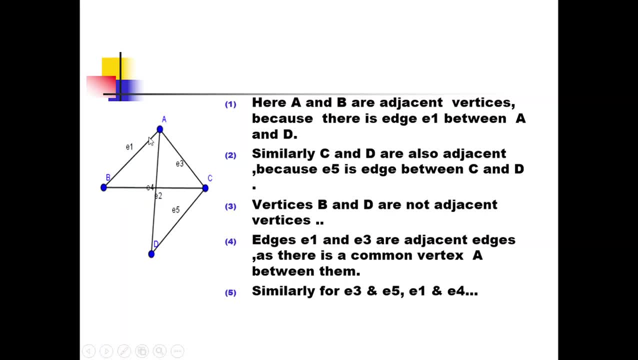 That is, connecting on those two vertex Means if you consider the example, That is example here. Here A and B are adjacent vertex Because they connect by the E1 edges. A and C is also adjacent vertex Because they connect by E3.. 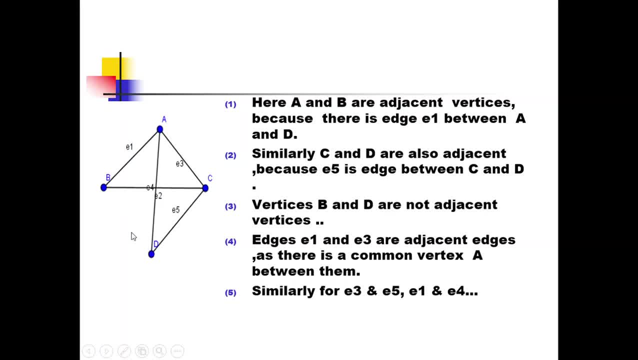 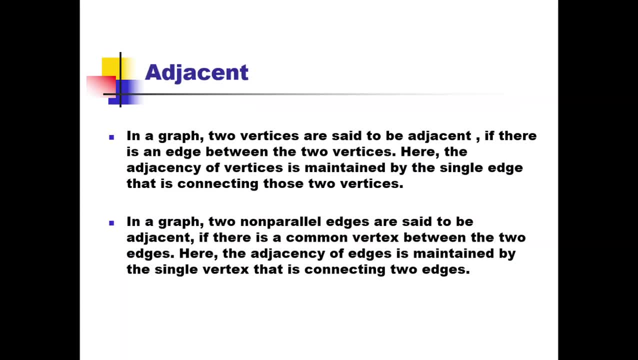 But B and D are not adjacent here Because that is not connect Directly here by single edge. So that is called adjacency to the vertex. Next is a adjacency to the edges. So what is meaning of that? In a graph, two non parallel edges are said to be adjacents. 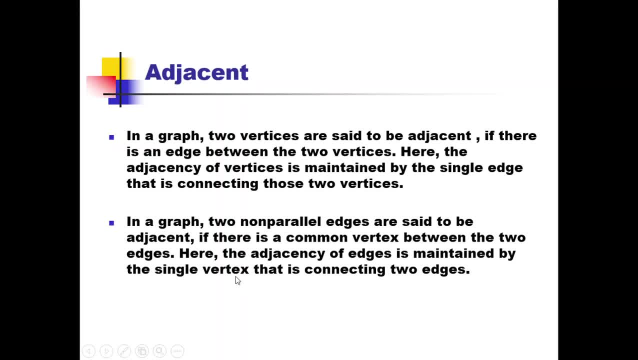 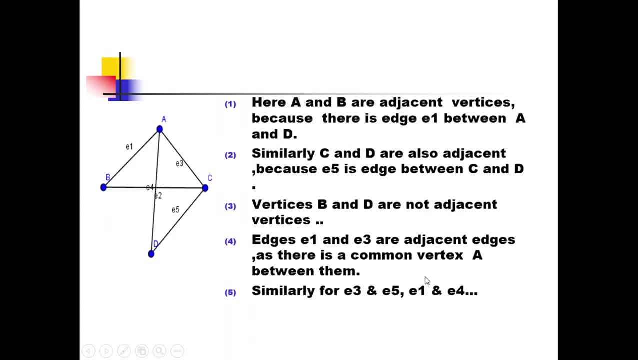 If there is a common vertex between the two edges, And here the adjacency of edge is maintained by the single vertex That is connecting two edges. So means in this graph E1 and E3 are adjacent edges Because that is connect by the single vertex A. 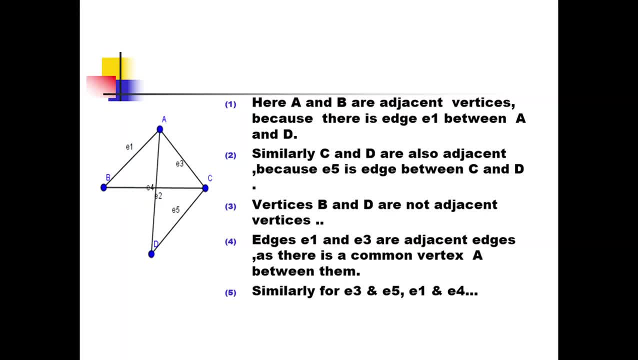 E1 and E4 is also adjacent here Because they connect by the single vertex. A, E3 and E5 is also adjacent edges Because they connect by the C. But E1 and E5 is not adjacent edges Because they not connect by the single vertex.